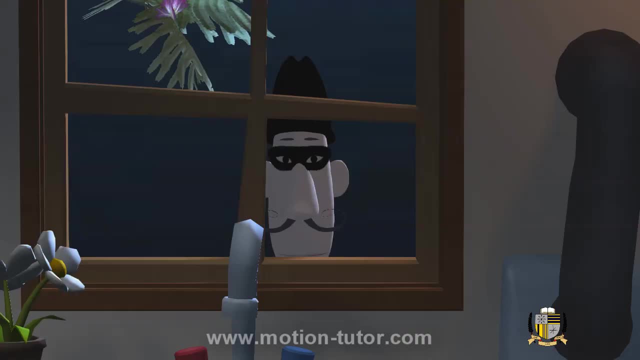 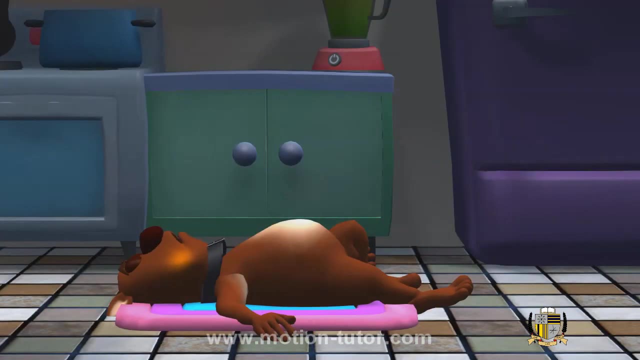 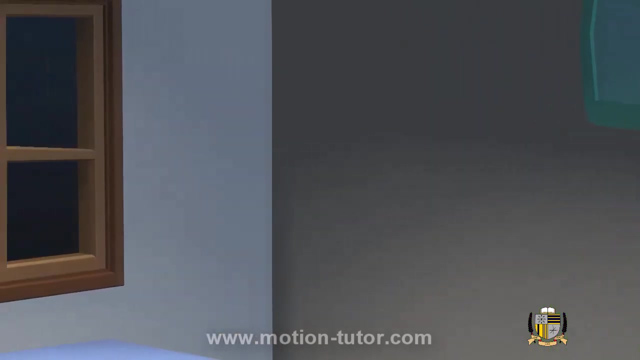 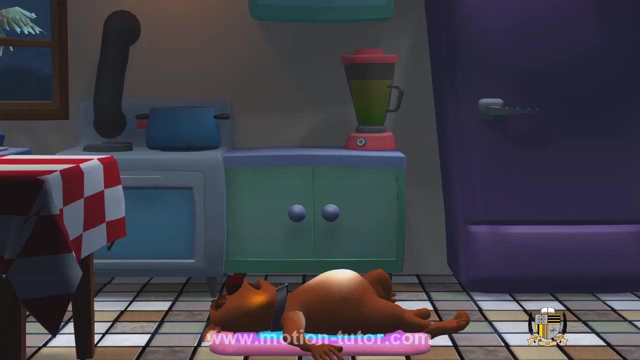 There are five cupcakes on the table. That guy outside wants to take away some. Let's see how he's going to do this. Meow Meow, I'm a cat. Meow meow, Meow, meow. 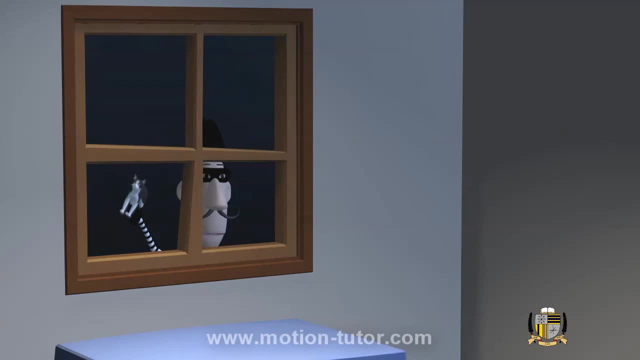 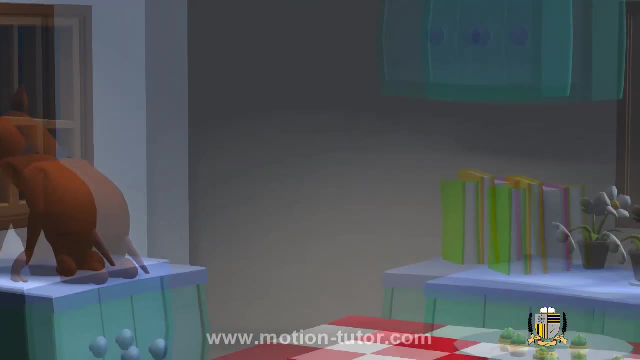 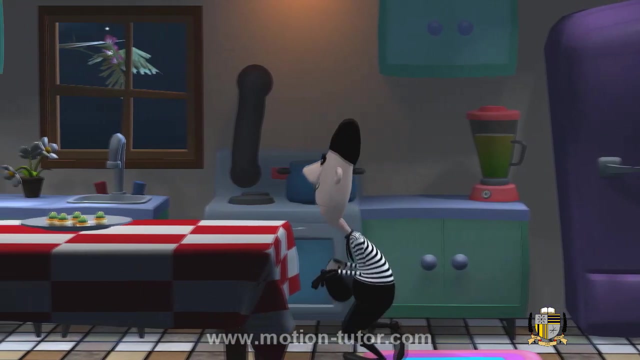 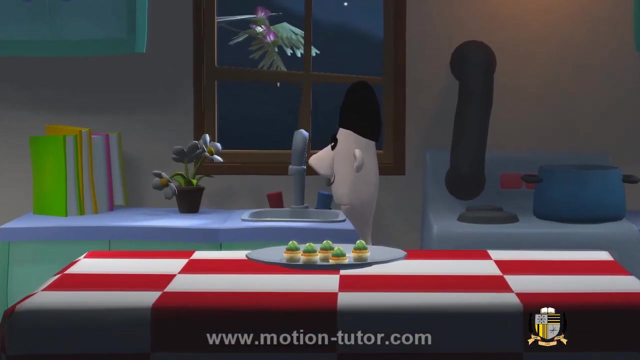 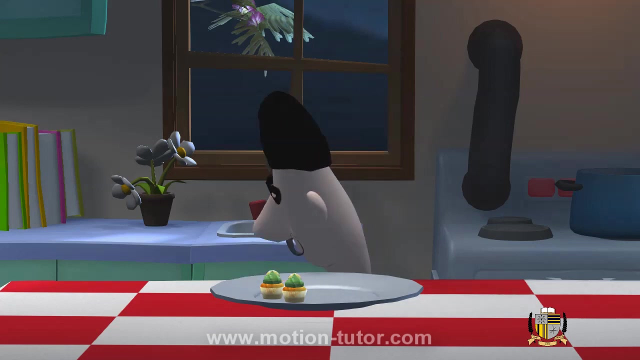 I'm a cat, Cat, cat, Meow, meow, Cat, meow, Meow, meow. OK, we saw him take away three cupcakes. Three cupcakes from the table. How many are still on the table? One, two. 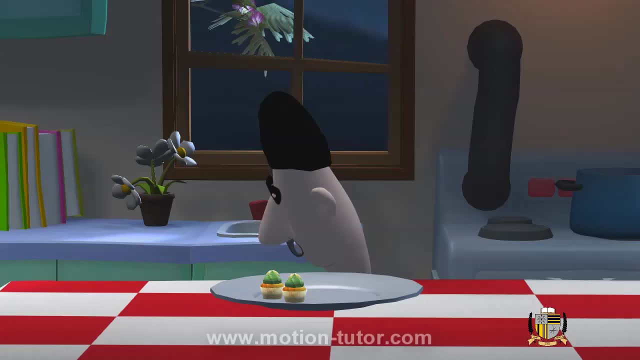 So five take away. three is two. Good job, sneaky guy. You can return those now, since you didn't ask for permission to take them. Shh, These are mine now, But that's not right. Ask for permission from the chef. 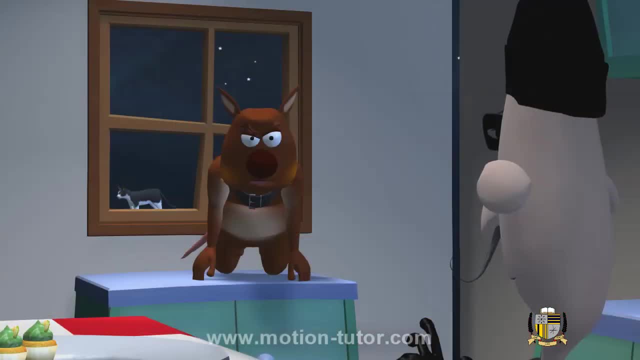 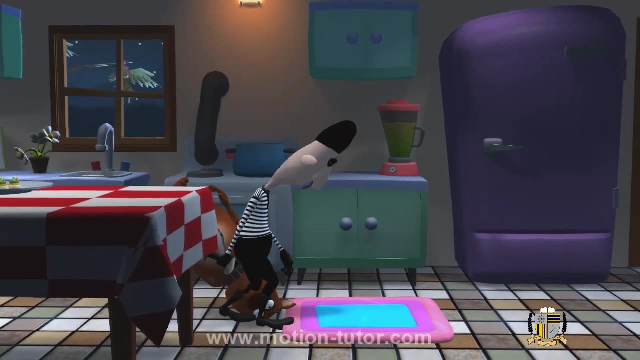 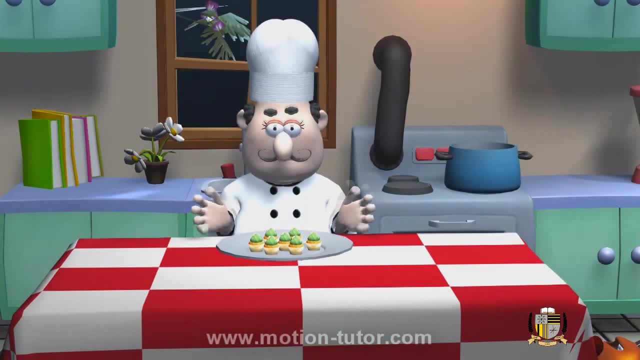 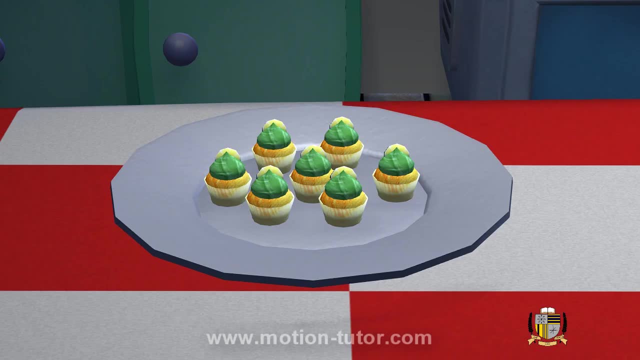 Yeah, Seven nice cupcakes for my guests tomorrow. They are seven cupcakes on the table. That guy outside wants to take away some. Let's see how he's going to do this. Meow, I'm a cat, Meow, meow.